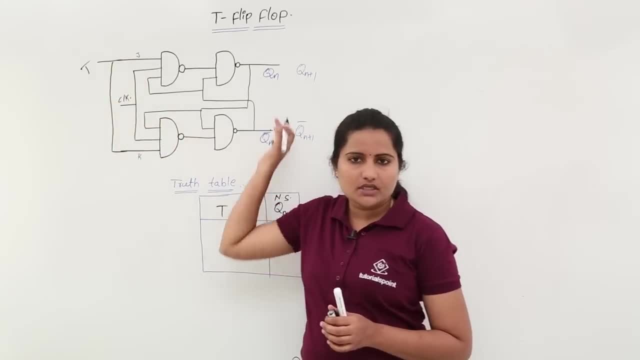 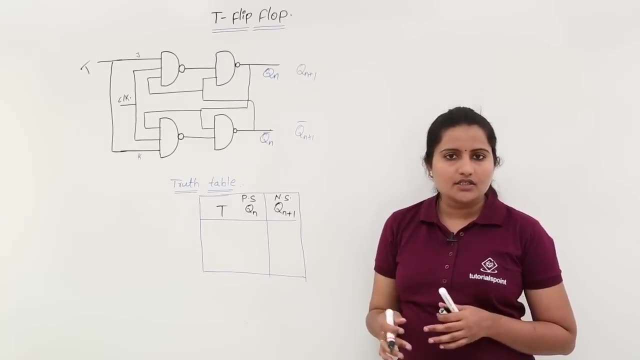 that means you can join J and K and you can use it as toggle flip-flop. it will provide only one condition. that means toggle condition, and other condition is no change. Obviously, T means you are having two inputs, either 0 or 1, in 0 condition. it will provide. 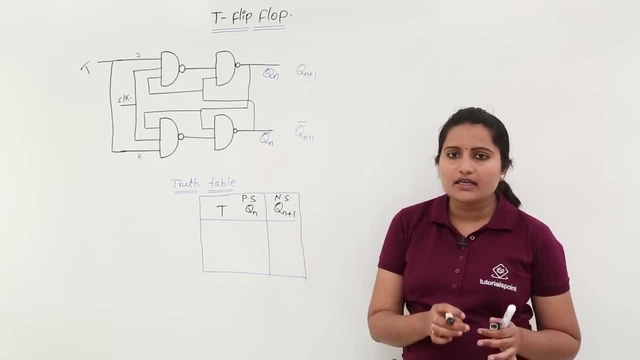 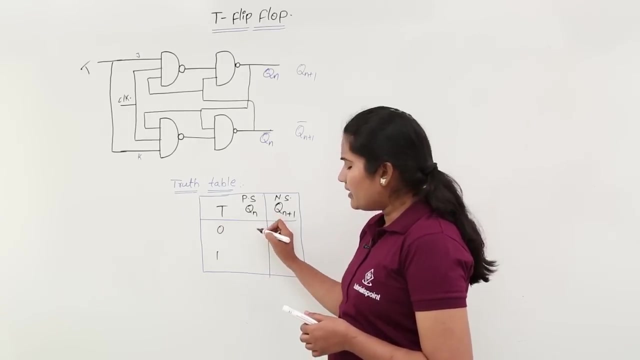 no change condition and if toggle is enabled, that means toggle is equivalent to t, is equivalent to 1. then it is going to provide our toggle output. So now we will see the operation here. So t may be either 0 or 1 here your qn. you do not know your present state, So 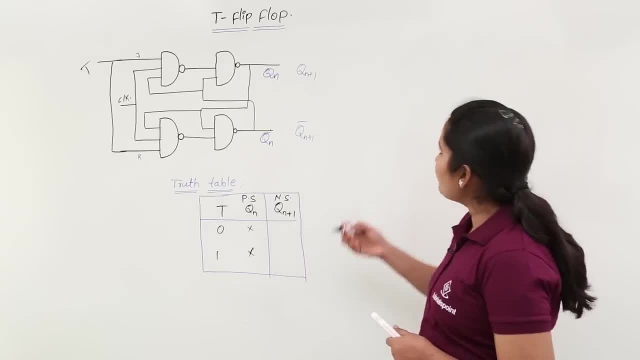 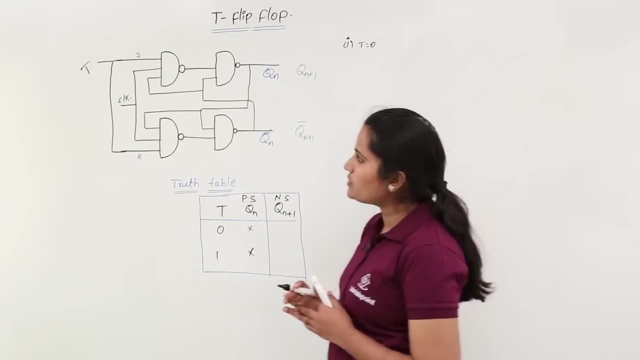 just now. just I am writing like do not care, So I am taking case 1.. So that case is equivalent to t equal to 0.. If t equal to 0, what is going to happen means every time clock must be is. 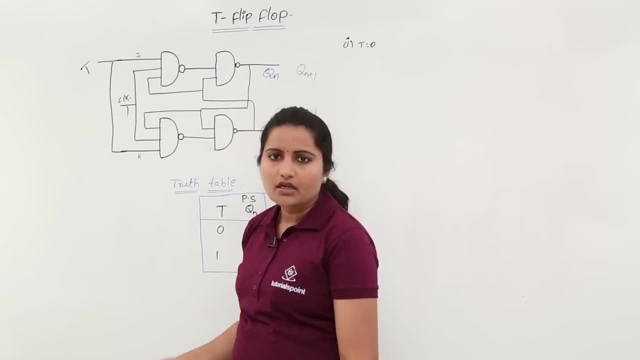 equivalent to 1, otherwise total flip flop will be in the same condition. So that is why I am taking clock as 1 to trigger my flip flop. So here, if t is equivalent to 0. So j equal to 0, k equal to 0 condition will take place. So here, when j equal to 0, k equal. 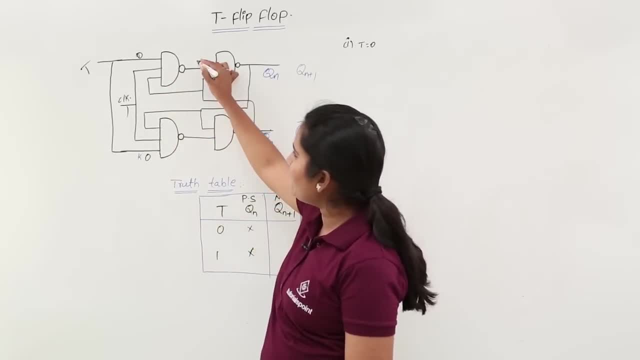 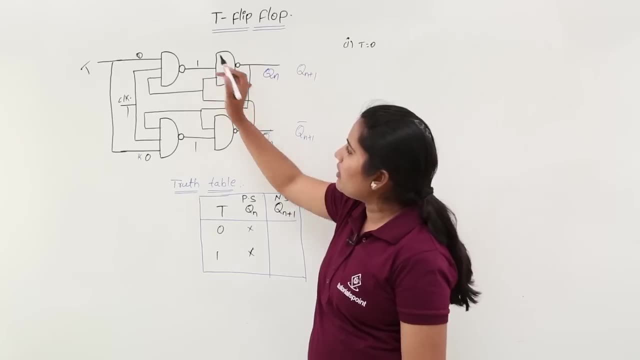 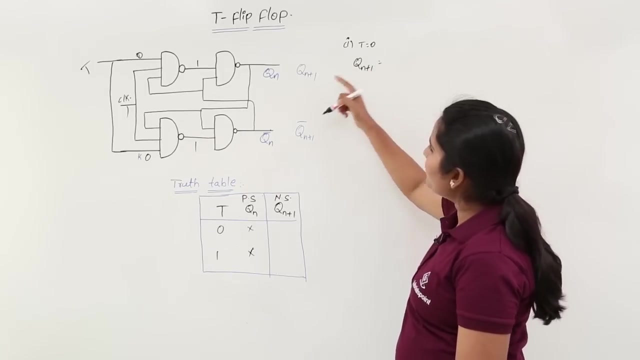 to 0. these two gates is going to provide 1, 1. As input of this latch circuit. So now here: if this gate output is equal n to 1, then I am just writing the equation for qn plus 1.. Every time you need to write equation for 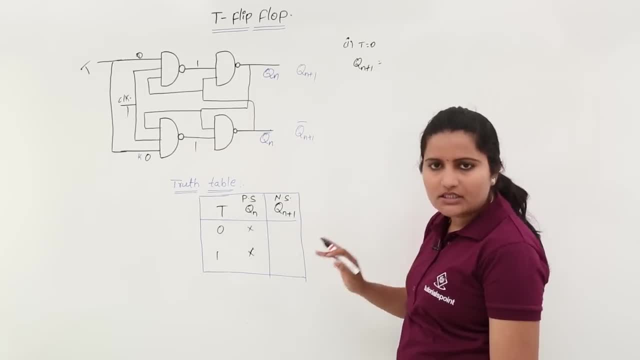 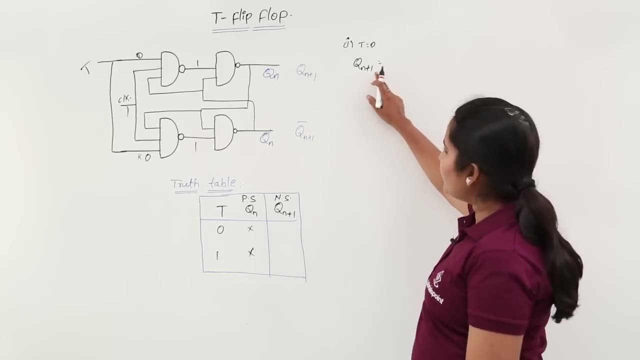 qn plus 1. these two are not outputs, these are just present states. Every time your output of your sequential circuit or flip flop is nothing but next state. So every time you need to write equation for qn plus 1 only by taking the reference, by bounding. So this: 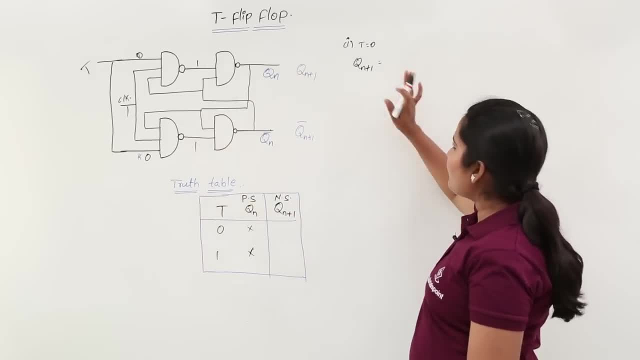 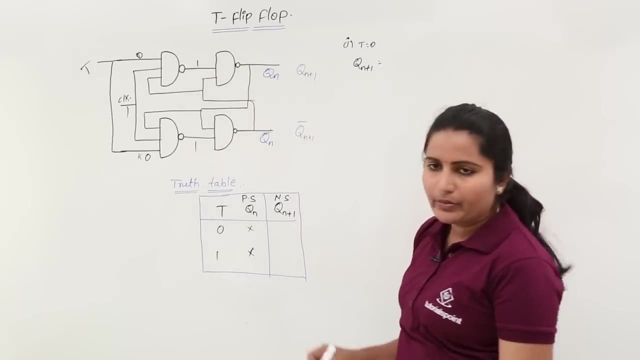 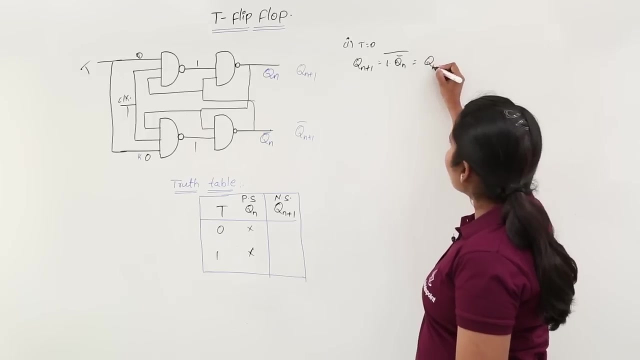 is the reference by back propagating these present states. So now I am writing qn plus 1 to get qn plus 1.. So I need this input from complement of present state, So 1 into qn bar, whole bar. you are getting here. you are getting qn, So you are not getting any. 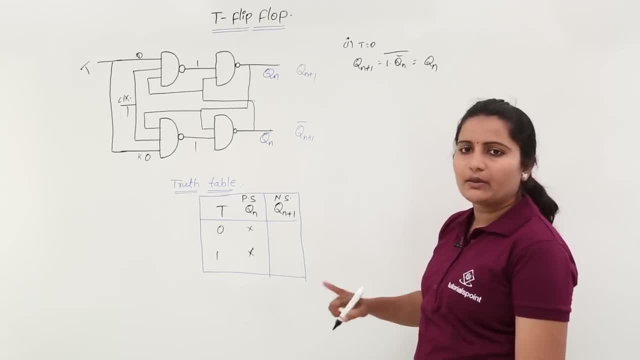 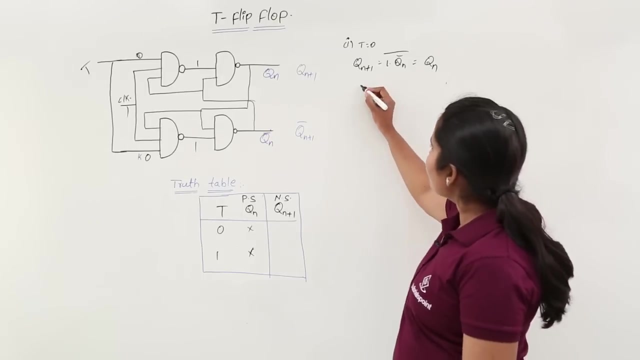 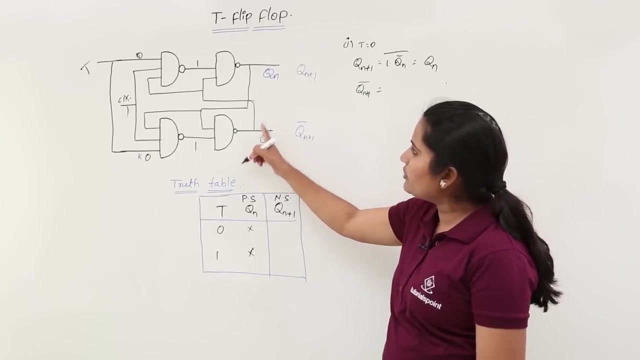 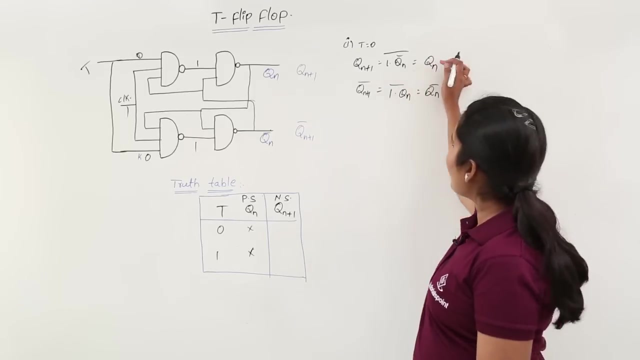 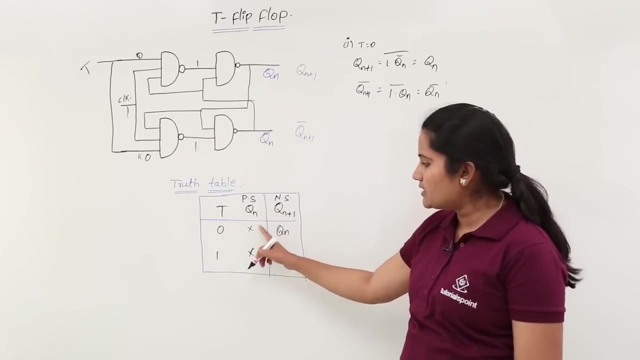 value. So that is why you need to check complement port also, whether you are getting value in complement port or not. So whatever value you got here that you can take here itself, So qn I am taking. So that means whatever qn is there, whatever present state is there, next state is also same only. 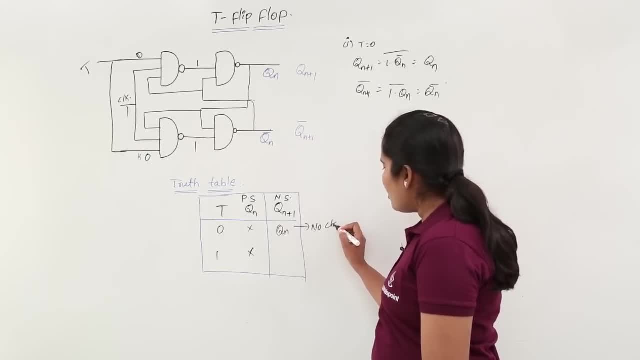 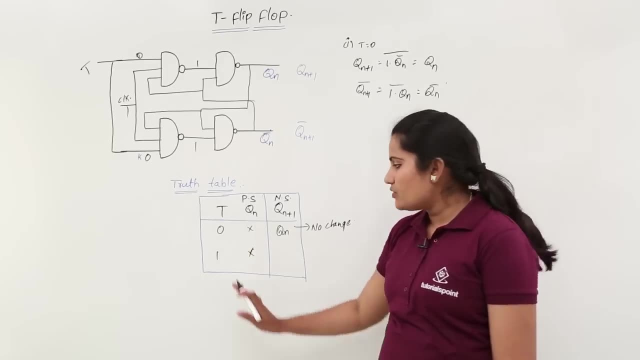 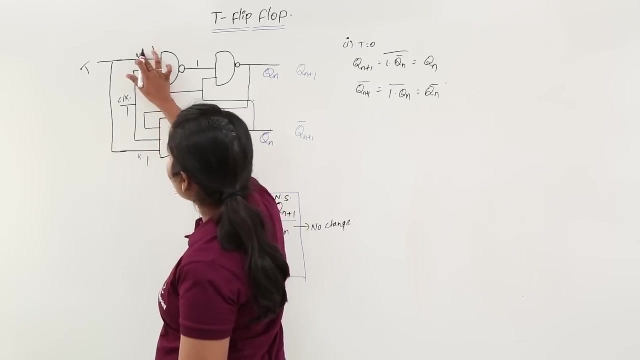 So this is called as no change condition of T flip flop. When no change condition in T flip flop will occur means when T equal to 0. So when T equal to 1, what is going to happen? means when T equal to 1. here you are providing 1, 1 in place of j k. So now, 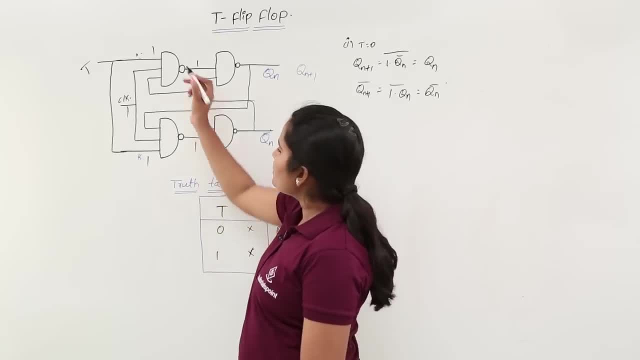 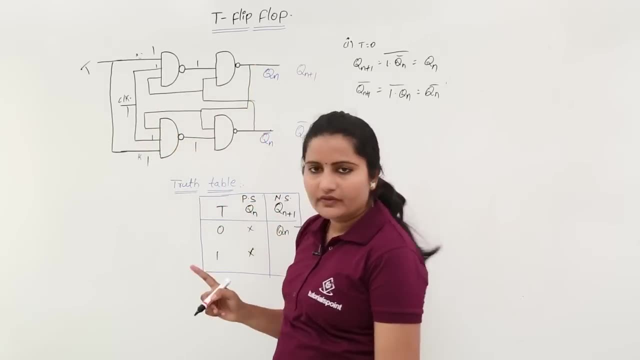 when these gates inputs are 1.. So see, here clock is 1 and here also clock is 1.. So here I am taking output of this gate 1 into 1 into So, this qn, So 1 into 1 into qn, whole bar. 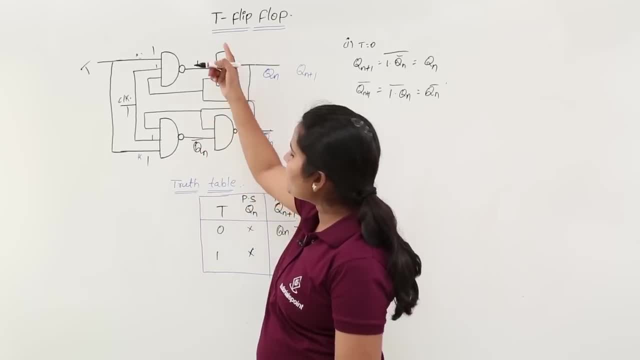 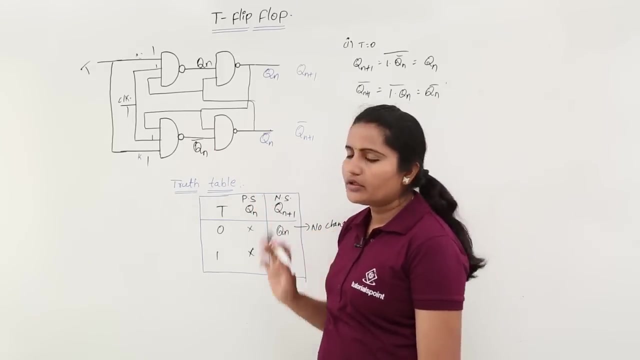 means here you are getting qn bar and top side. you are getting 1 into 1, into qn bar, whole bar. here you are getting qn. you can see. Now I am just taking this qn to output. that means you can take 0, 1 or 1, 0 you can take. 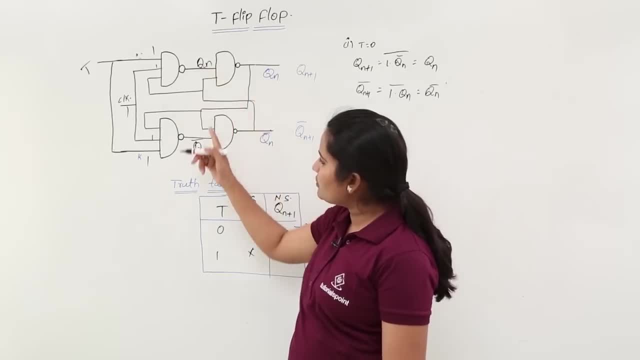 0, 1 or 1: 0.. So q, if qn equal to 0, qn bar, you are getting 1.. For example, if you got 0 here, obviously you are getting 1 here. Then what is the output you are getting? what is the? 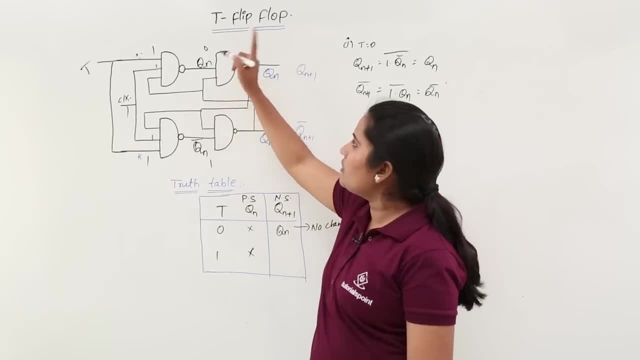 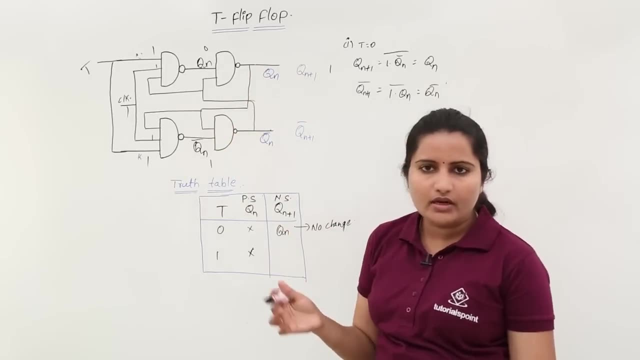 qn plus 1. you are getting that means 0 into anything whole bar. you are getting 0 into 0. So you are getting 1 here and here you are getting 1 into. So qn whole bar, whatever you are having that you are getting. So whenever you are having 0, you are getting 1 as qn plus. 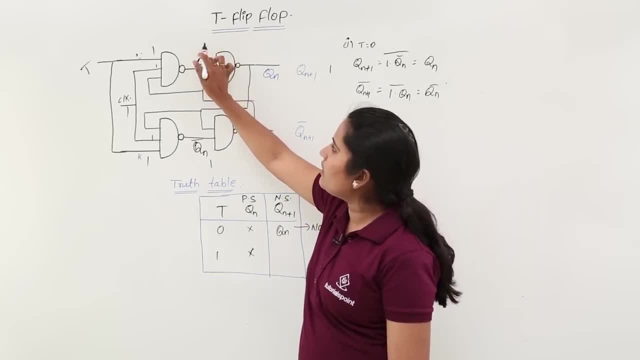 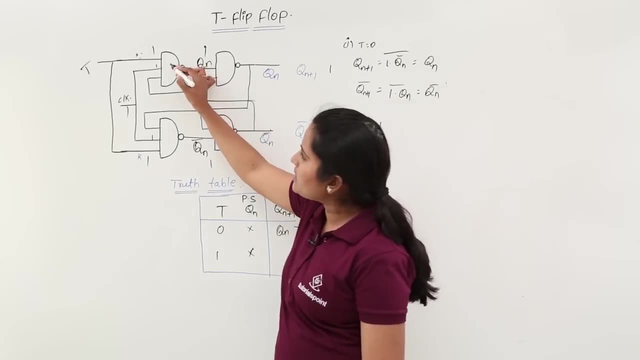 1.. For example, qn is equivalent to 1. you can consider here In this case, when T is equal to 1 after processing. you just consider, these gates are g 1, g 2, g 3 and g 4.. So my 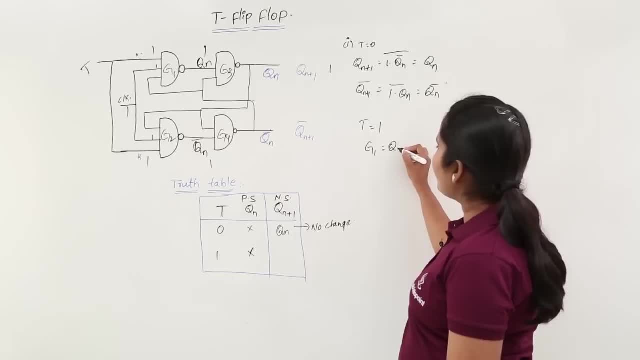 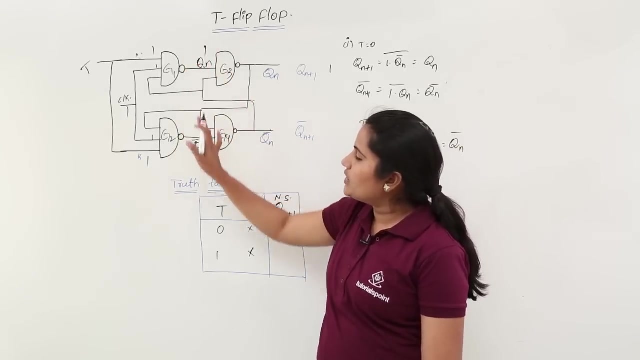 g 1 output is equivalent to qn and g 2 output. you are having qn bar. I am just considering qn is equal to 0, qn may be 0 or 1.. The 2 possibilities of these 2 inputs may be 0, 1 or 1: 0 because 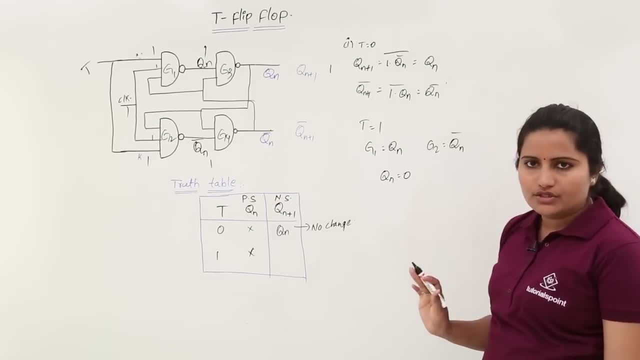 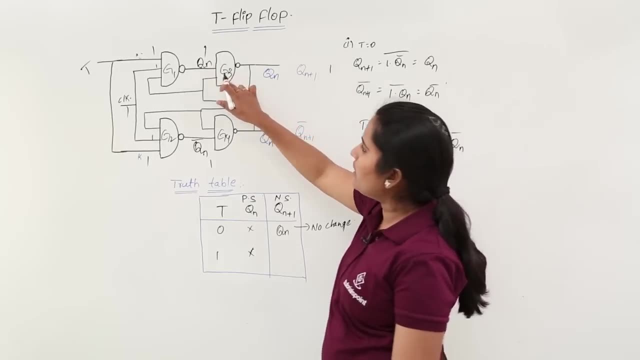 we are having complement, For example, qn equal to 0, then what you are getting at qn plus 1.. Q n equal to 0 means 0 into anything bar you are getting. Q n plus 1 is equivalent to 0. 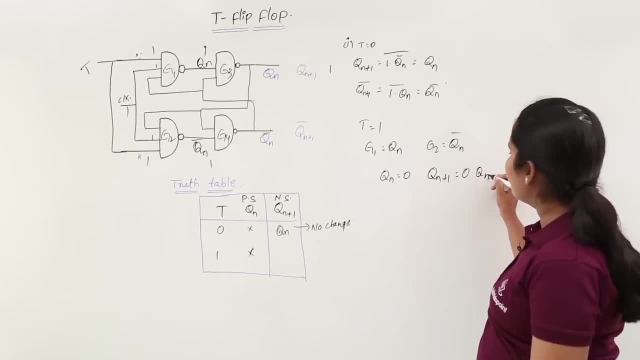 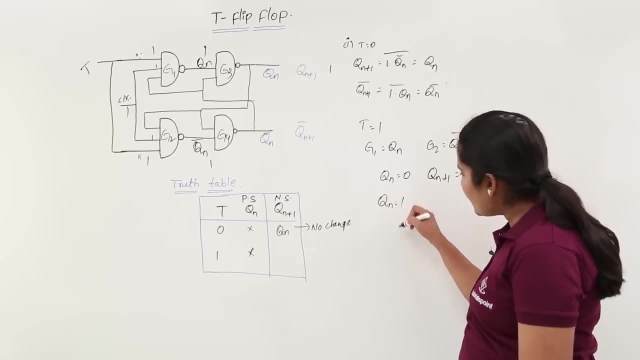 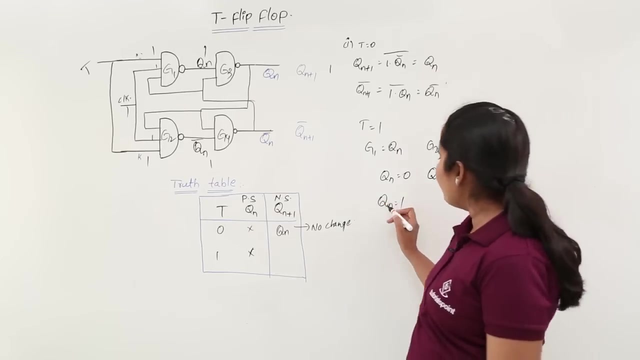 into so that Q n bar, whole bar, is equivalent to. you are getting 1 here. Now, for example, Q n. if you considered 1, you got 1 in place of Q n. So then what you are getting means so if Q n is equal to 1, you can see this port. 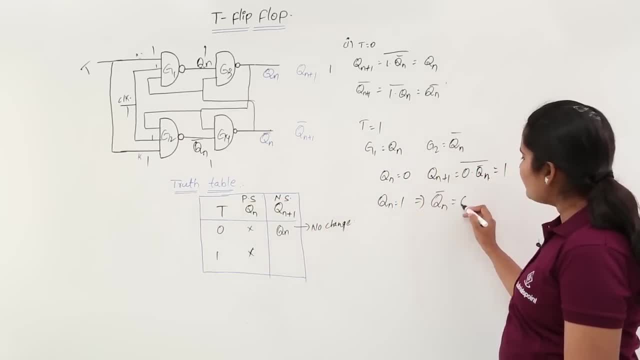 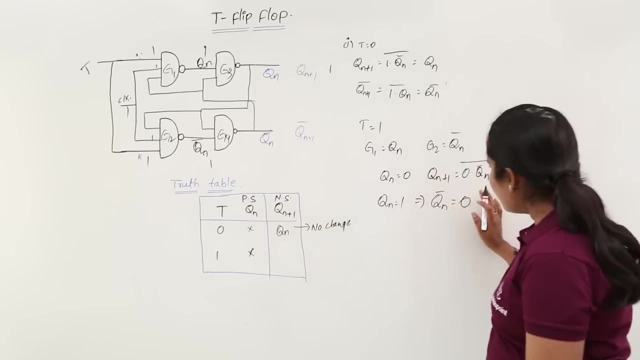 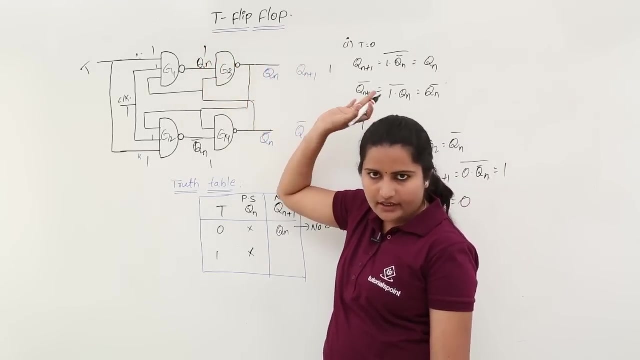 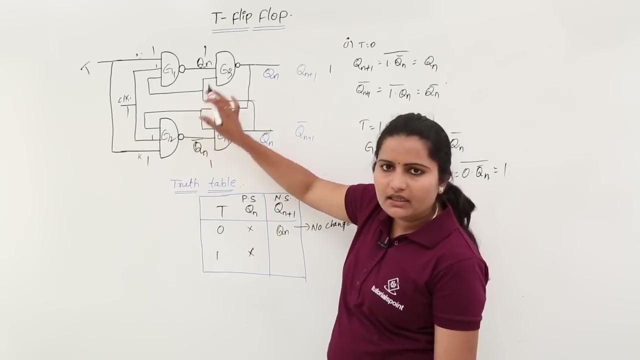 Q n bar is equivalent to 0. I am operating this port because this is easy. So see here: when Q n equal to 0, it is better to operate this gate because 0 into anything, 0 bar, you can take 1.. Now in the second case, Q n is equal to 1.. So this case is better than dealing. 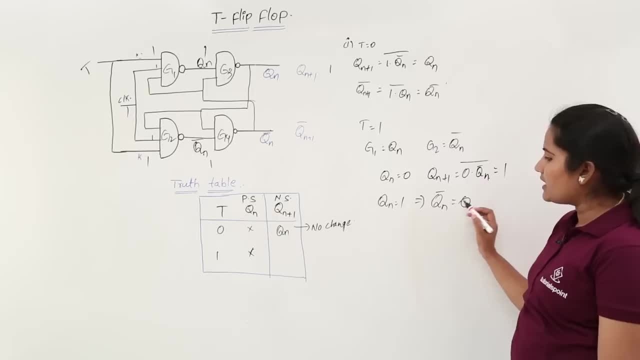 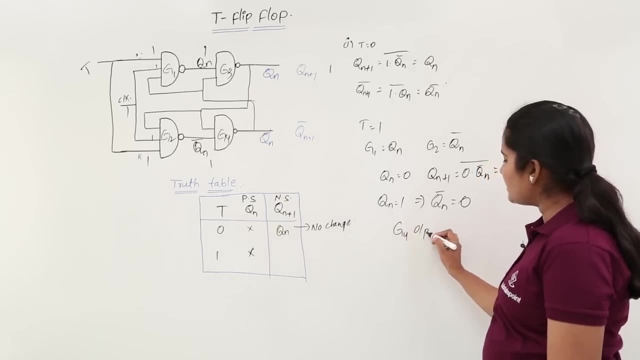 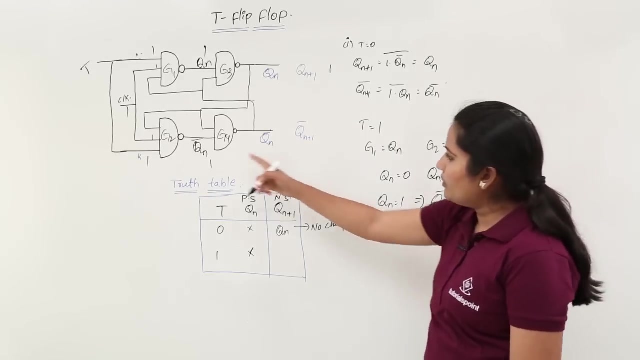 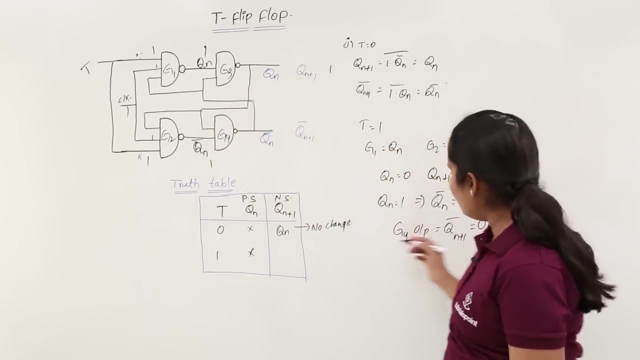 this case first. thus that means Q n bar is equal to 0.. So here 0 into G 4 output. G 4 output- I am considering G 4 output- is equal to Q n plus 1 bar is equivalent to So here. so Q n bar means Q n bar is 0 into and another input is Q n. 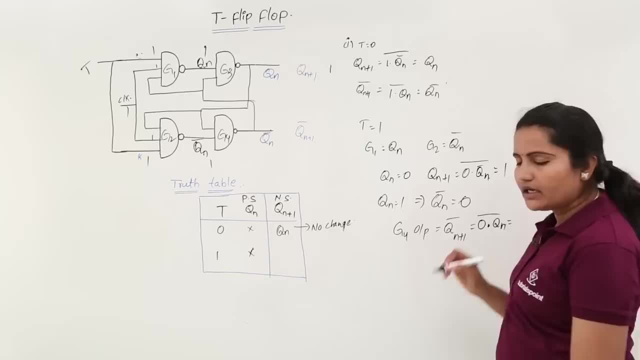 So another input is Q n whole bar is equal to 0 into anything. whole bar means you are getting 1.. That means Q n plus 1 bar you are getting as 1 means. So that implies Q n plus 1, you are getting 0.. 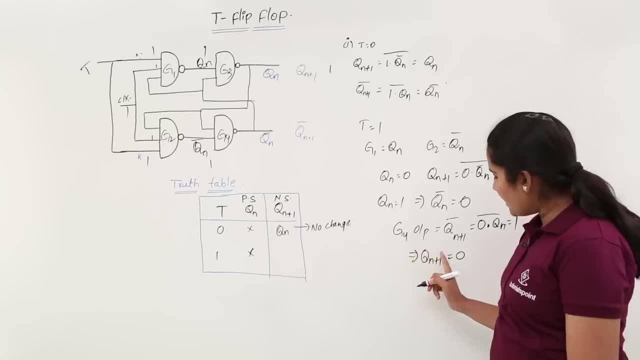 So, complement of Q n plus 1, you are getting 1, means Q n plus 1, you are getting 0. That means you can observe these two cases: when Q n is equal unto 0, you are getting Q n plus 1 as 1.. 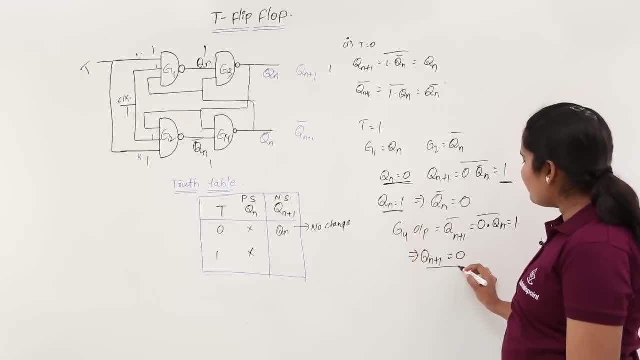 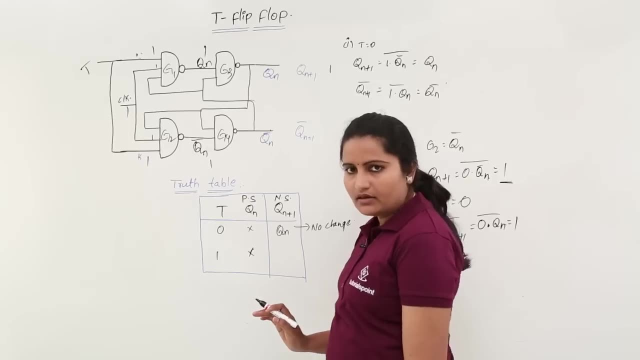 When Q n is equal to 1, you are getting Q n plus 1 as 0 complement of that. So that means so, whatever Q n plus 1 is there, That Q n plus 1, you are getting complement to Q n bar. 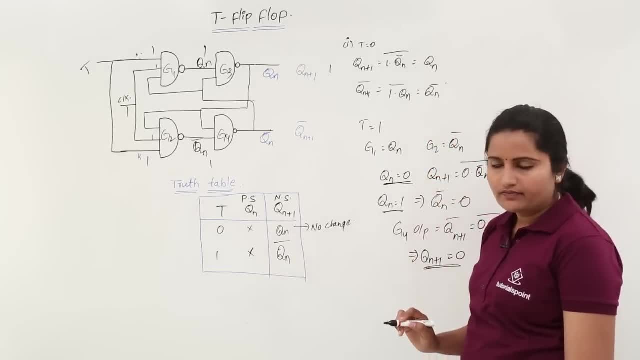 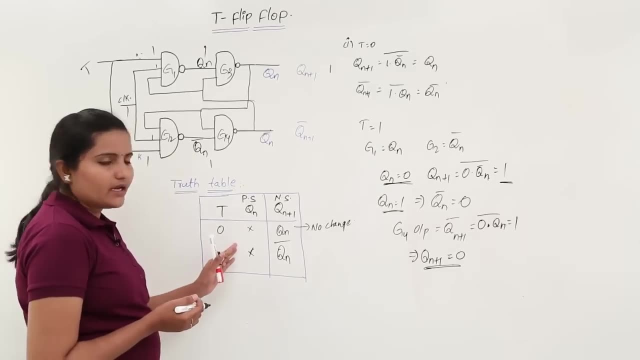 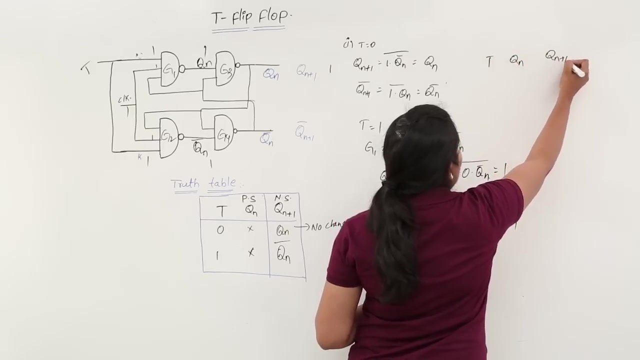 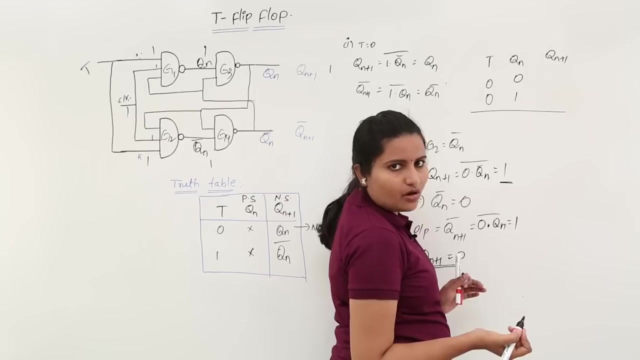 So here I am writing like this: So now, if you want expression for T flip flop, then what you are doing is simply, I am just enlarging this truth table. So that means T, Q n, Q n plus 1.. So in 0 case of T, your Q n value may be either 0 or 1.. 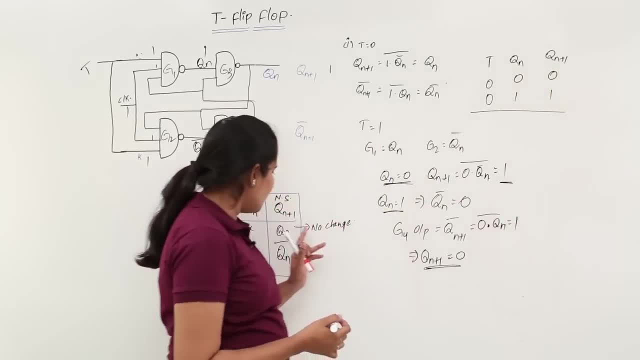 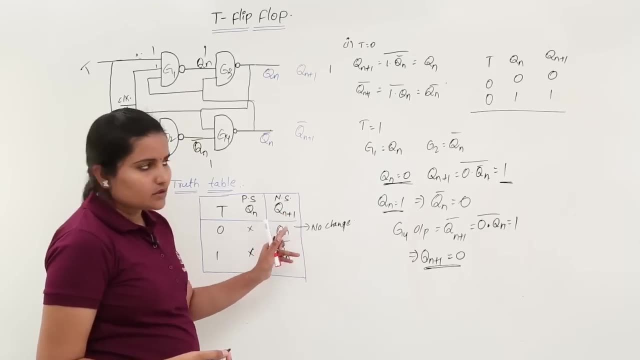 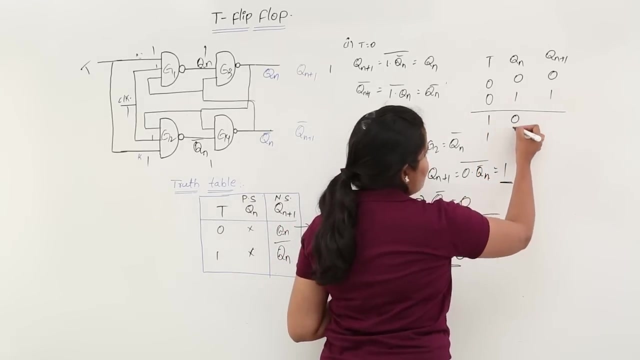 So in this case you are getting equivalent to Q n. So Q n is either 0 or 1. that same Q n you are getting at output port. So I written like this: In case of T equal to 1, the Q n may be either 0 or 1, you are getting complement of Q n. 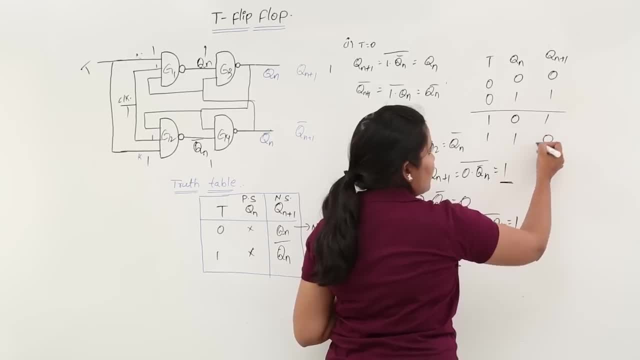 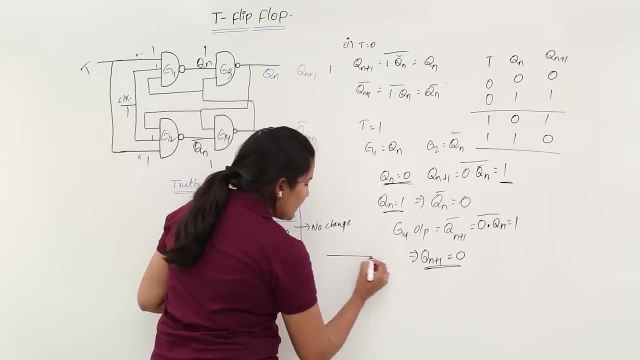 That means when 0 is there, you are getting 1. when 1 is there, you are getting 0.. This is the expanded truth table. Now this is the time to draw K. How many variable K map? you need to consider means. 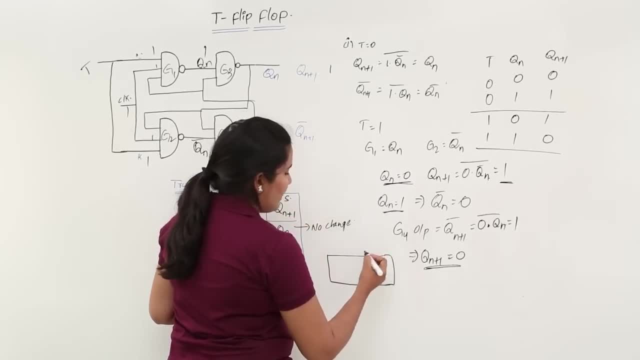 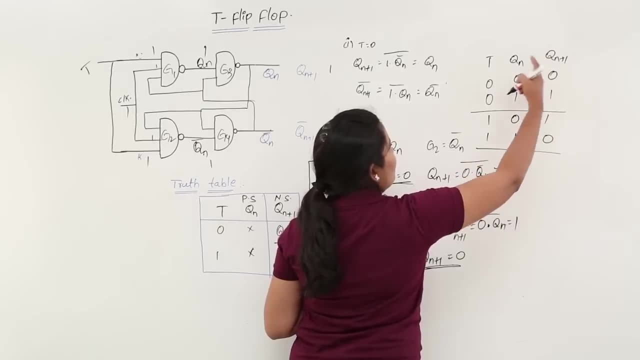 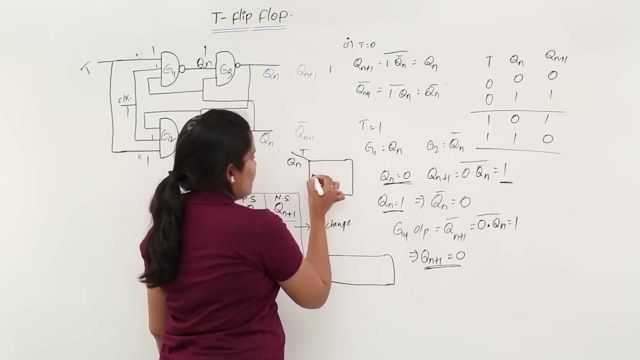 So I am considering 2 variable K map. Why? because this is enough to consider 2 variable K map here. because for this output the 2 possible inputs are T and Q n only. So I am considering Q, n and T like this simple T variable K map. I take in where you are having. 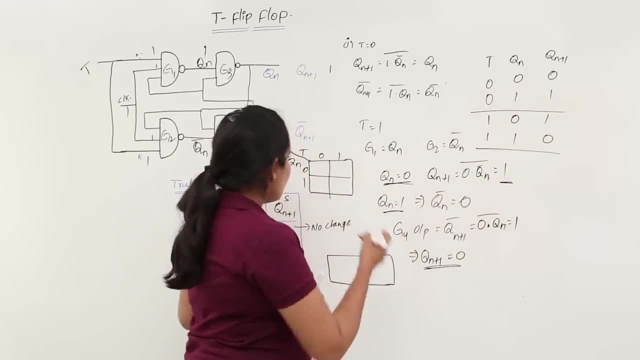 your 1's means at T 0, Q n 1.. At a T 0, Q n 1 and at a T equal to 1 and at a T equal to 1 and Q n equal to 0.. T equal to 1, Q n equal to 0 means here: